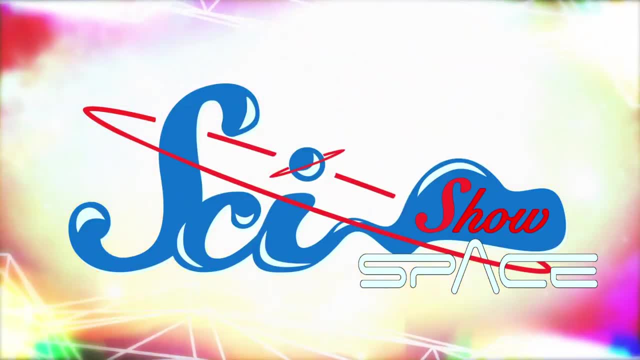 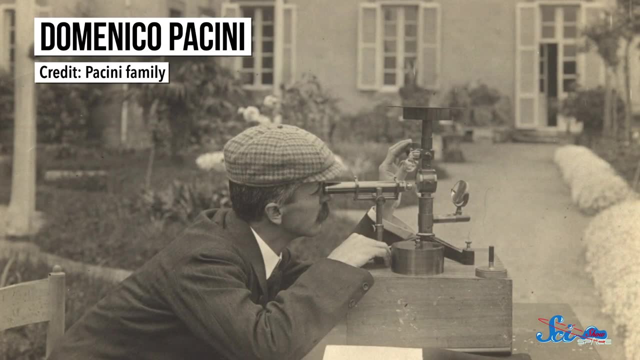 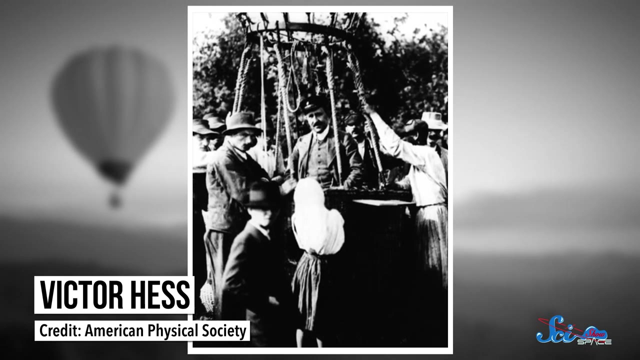 Around 1910, two small but mighty experiments popped up in the scientific literature. The first was from a physicist named Domenico Pacini in 1911. He set instruments underwater and measured radiation levels at different depths. The second came from another physicist named Victor Hess. 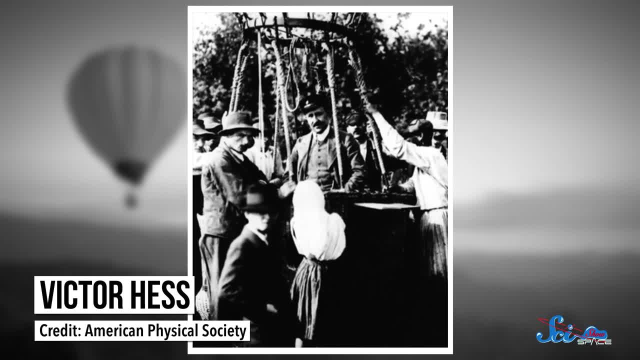 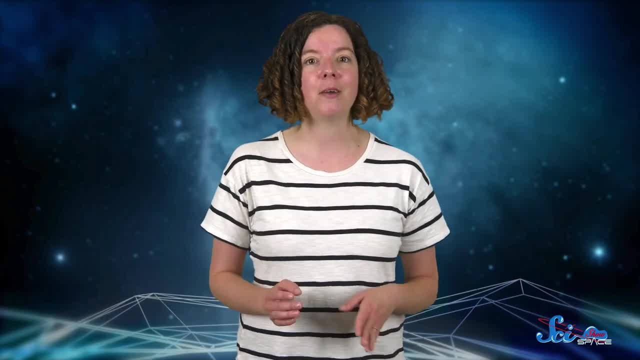 In 1912, he jumped in a hot air balloon and traveled about 5 kilometers above Central Europe to measure the radiation way up there. These experiments might seem like standard data-collecting stuff, but they helped reveal something that would change the way we understand the universe. 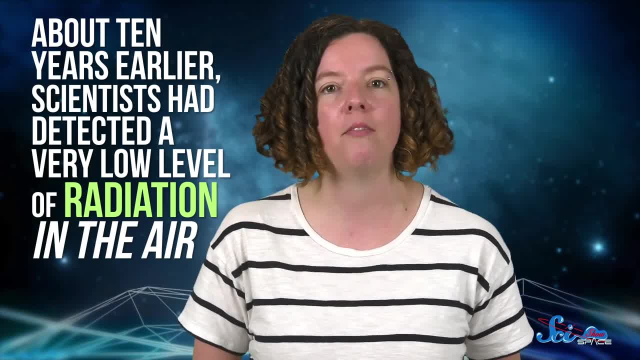 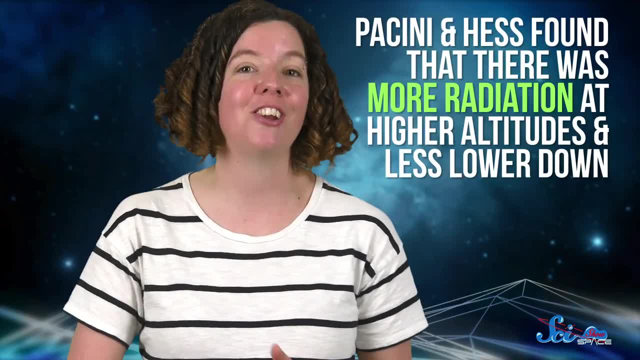 See: about 10 years earlier, scientists had detected a very low level of radiation in the air. Originally they assumed it came from rocks, but Pacini and Hess showed them that they were wrong. They found that there was more radiation at higher altitudes and less lower down. 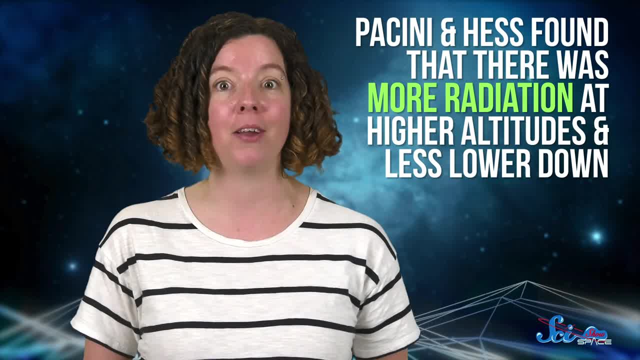 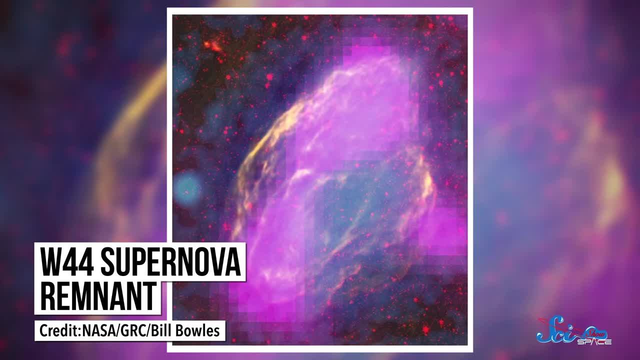 And that meant that radiation couldn't just come from the Earth. Some of it had to be coming from space. Eventually, this kind of radiation became known as cosmic rays. Today it's mostly used to understand the objects that produce it, but in the early 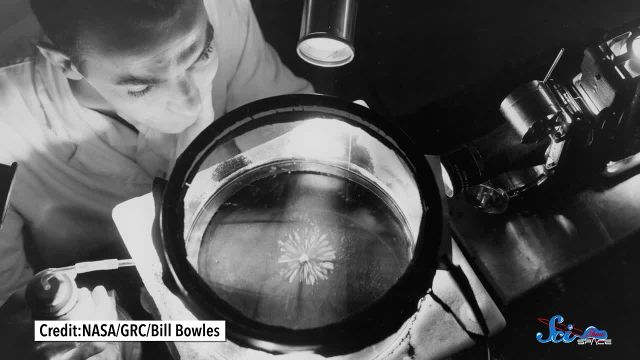 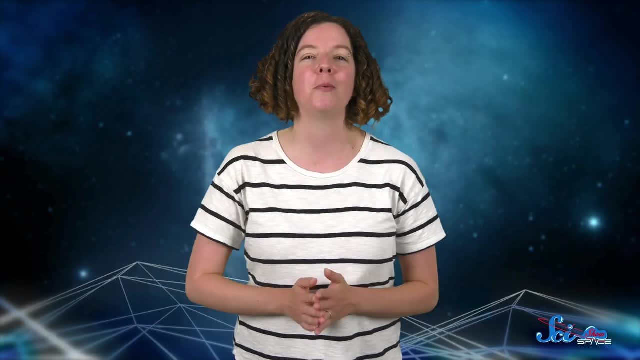 1900s it had a different job. It helped us discover brand new subatomic particles long before today's accelerators were a glimmer in any physicist's eye. So in a way, all those experiments underwater and in balloons didn't just help us find. 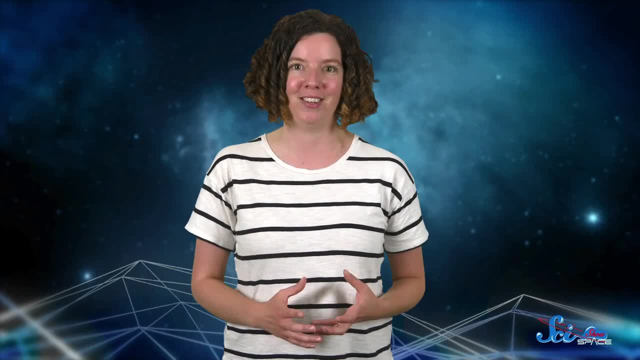 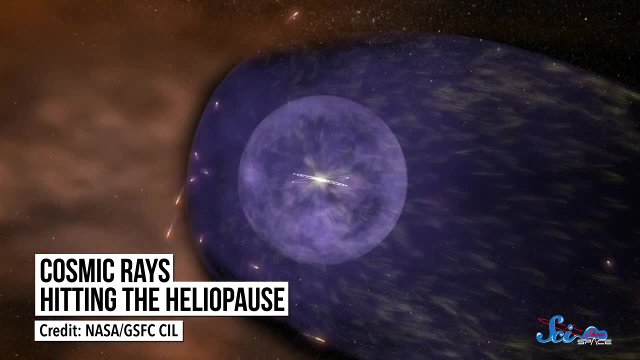 some space radiation. They helped found modern particle physics. After we first discovered them it took decades to figure out what cosmic rays were, But today we know they're charged particles that are constantly hitting Earth at nearly the speed of light. They're mostly made of individual protons but have a few electrons and larger atomic. 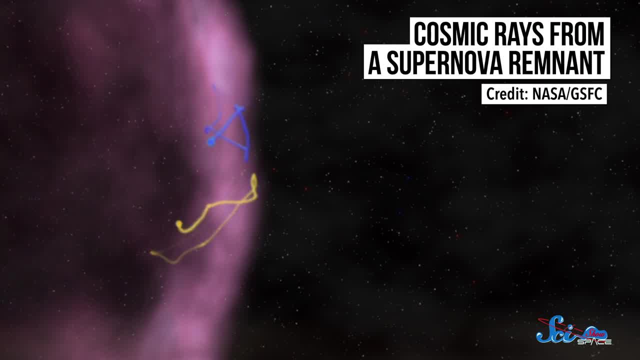 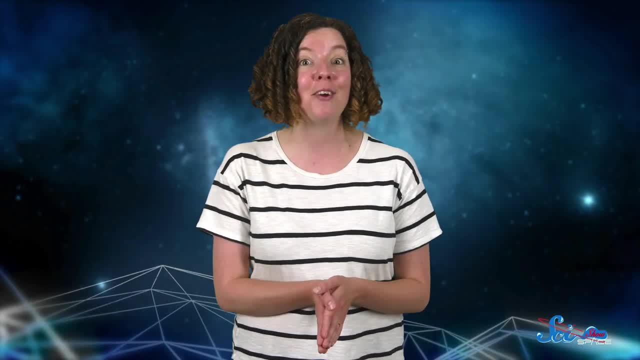 nuclei every once in a while too, And while some come straight from the Sun, most of them don't. Most are from big destructive things like supernovas or stars falling into black holes. Recently, astronomers have used these rays to learn about these extreme environments. 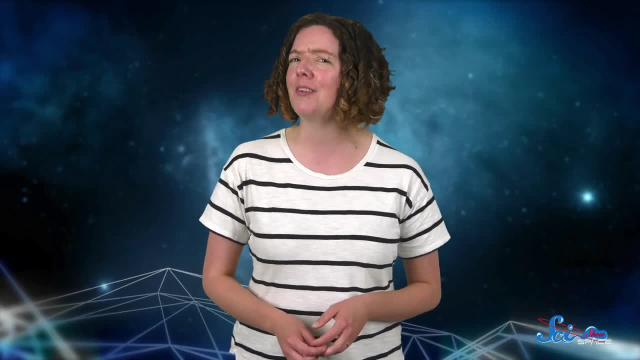 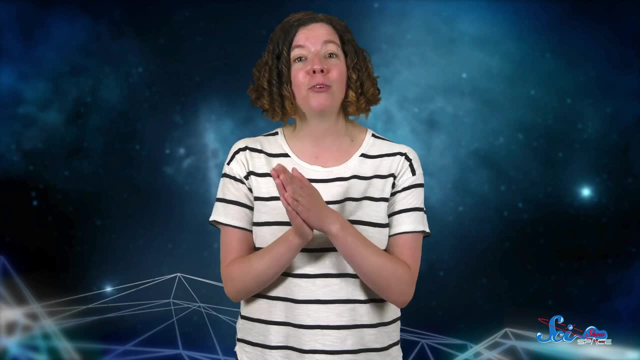 But many scientists in the early and mid-1900s weren't really focused on the rays themselves. Instead, they studied what happened when cosmic rays reached Earth. And good thing they did, because these rays ended up being one of our most important early 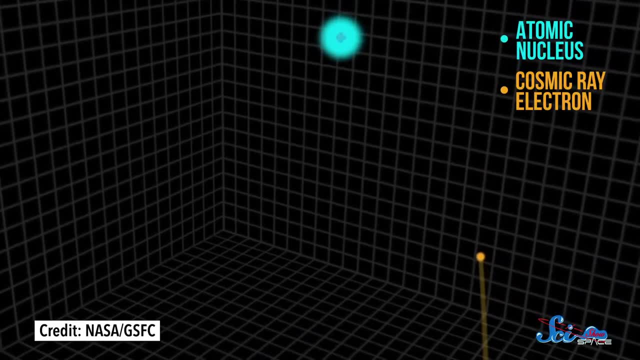 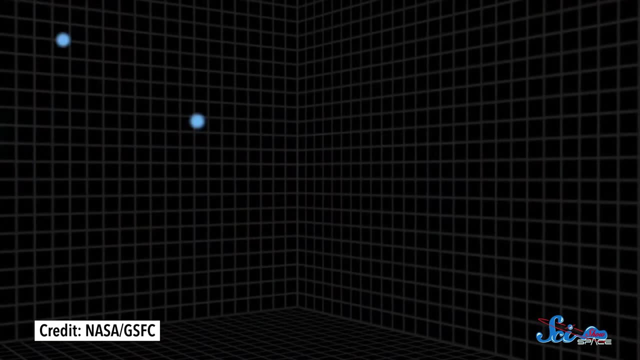 tools for studying the universe. Since cosmic rays move very close to the speed of light, they carry a lot of energy. When they hit things, that collision is so powerful that the energy itself can't be turned into subatomic particles. The idea that energy and matter are interchangeable is actually the whole point of E equals mc squared. 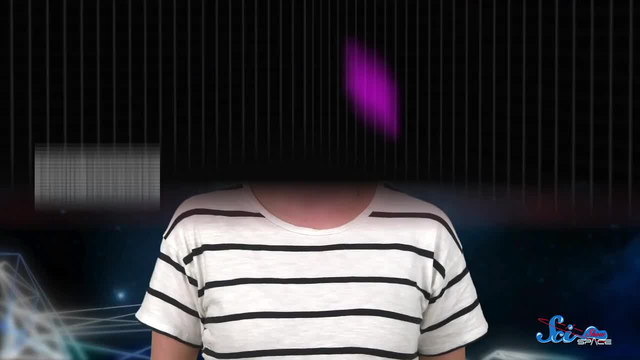 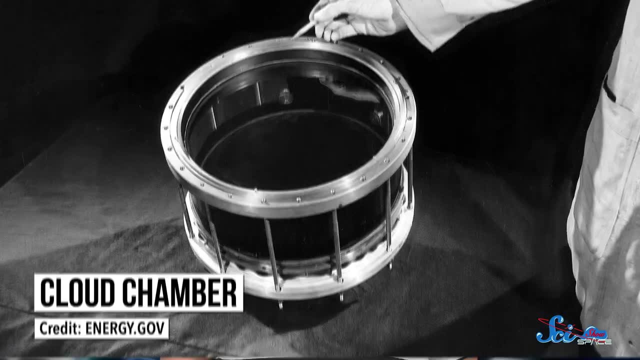 so the energy-becoming-particles thing isn't game-breaking, But it was game-changing because some of the particles that popped up in those cosmic ray collisions were things we had never seen before. In the early 1900s scientists were able to study them in devices called cloud chambers. 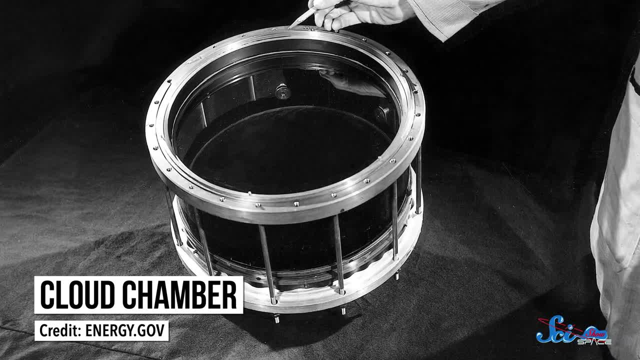 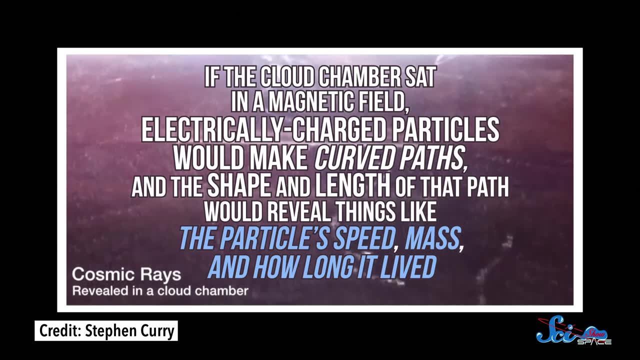 where water or alcohol vapor condensed into a cloud around anything that passed through it. They watched how the particles moved in these chambers, and then they could use that data to figure out their properties. For instance, if the cloud chamber sat in a magnetic field, electrically charged particles 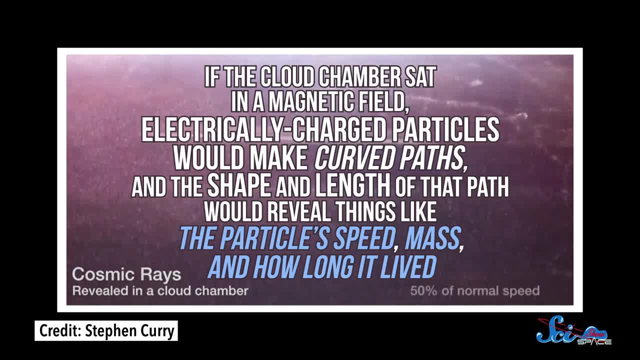 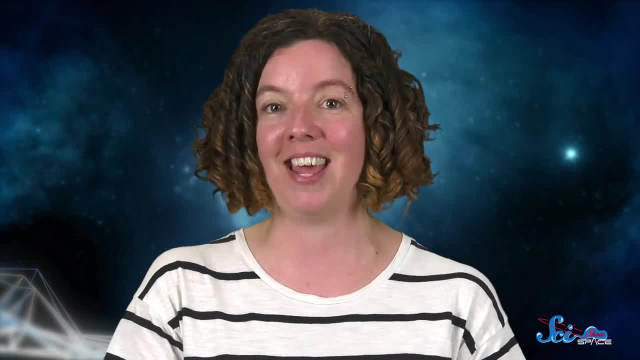 would make curved paths And the shape and length of that path would reveal things like the particle's speed, mass and how long it lived, Which sounds like magic, but it's actually a pretty straightforward research method and it revealed so much. 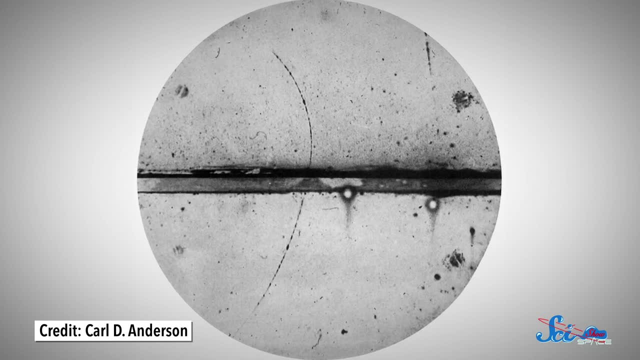 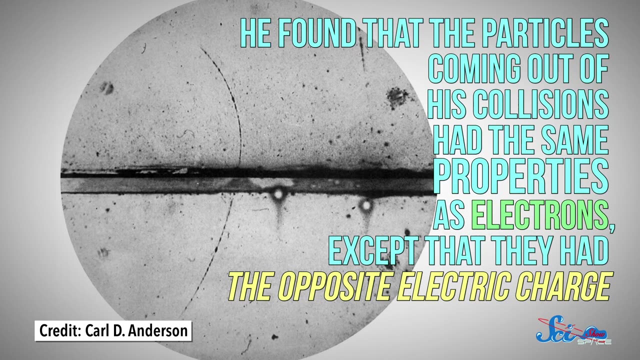 In 1932,, for example, a post-doctoral researcher named Karl Andersen was using these sorts of methods to watch cosmic rays hit a lead plate. He found that the particles coming out of his collisions had the same properties as electrons, except that they had the opposite electric charge. 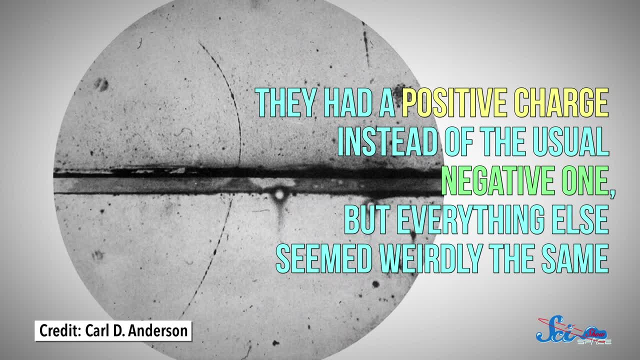 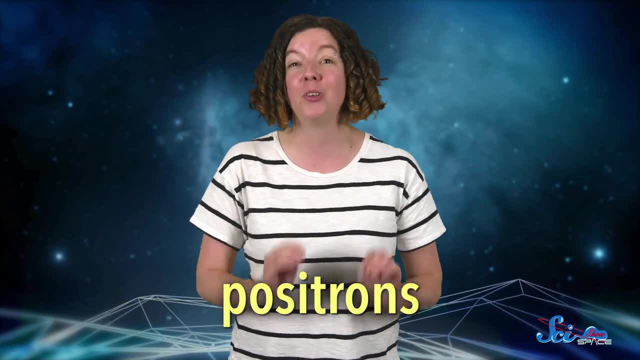 They had a positive charge instead of the usual negative one, but everything else seemed weirdly the same. As it turned out, Andersen had discovered positrons and the first kind of antimatter ever observed. All matter has an antimatter counterpart, so Andersen effectively doubled the number. 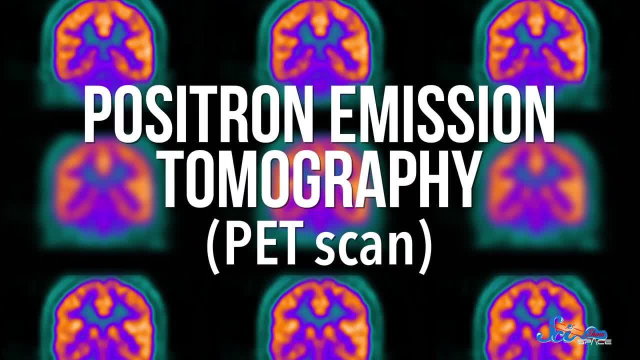 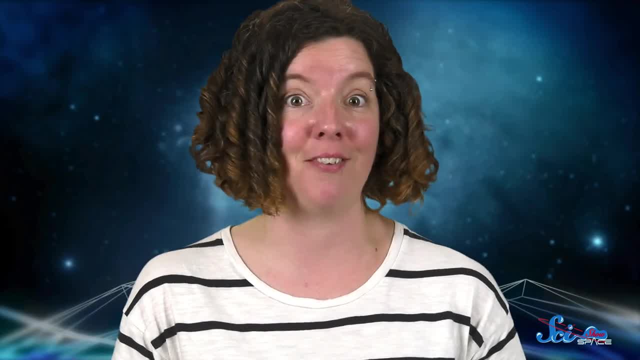 of known particles with a single discovery, And if you know anyone who's ever had a positron emission tomography or PET scan, you can thank Karl Andersen. But that wasn't his last cosmic ray discovery. A few years later, he and others found another key particle, the muon. 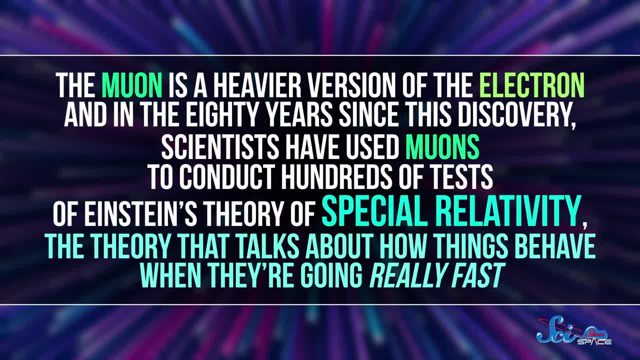 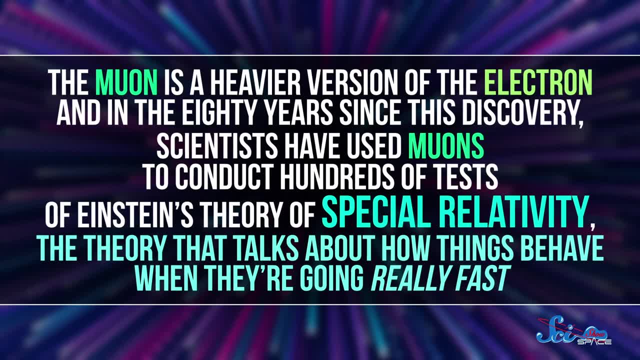 It's a heavier version of the electron and in the 80 years since this discovery, scientists have used muons to conduct hundreds of tests of Einstein's theory of special relativity, the theory that talks about how things behave when they're going really. 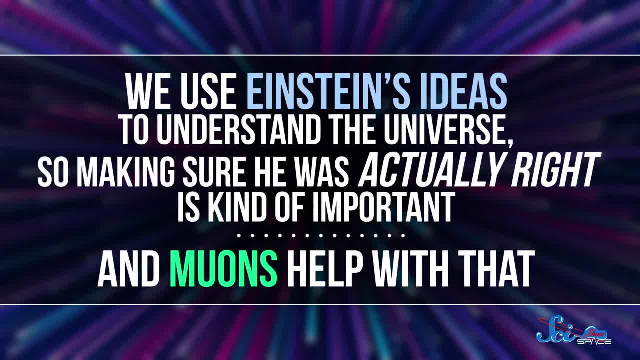 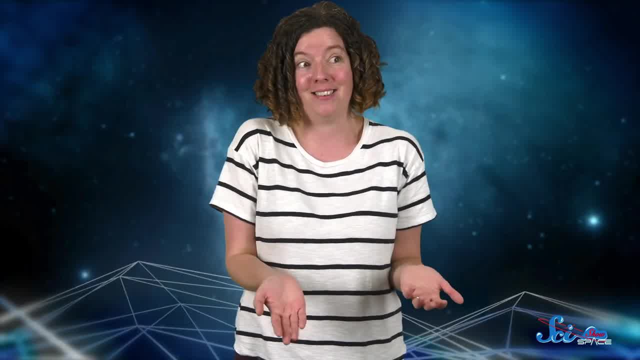 fast. We use Einstein's ideas to understand the universe, so making sure he was actually right is kind of important, And muons help with that. But in the 1940s the most important thing about muons was that they existed. 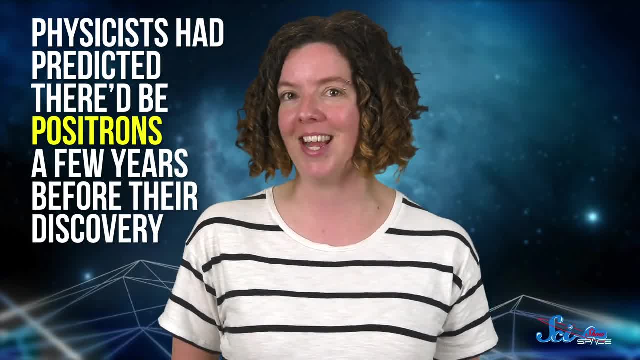 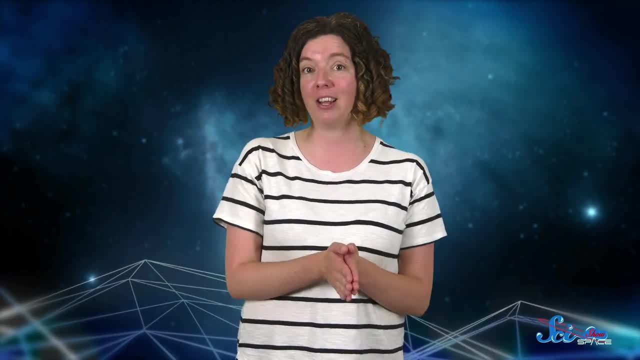 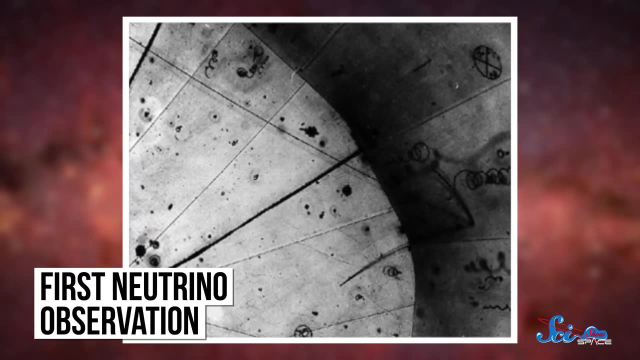 They were completely unexpected, and the closer physicists watched cosmic ray collisions, the more of these sorts of surprises popped up. They even put scientists on a path that would lead to the discovery of quarks, the tiny building blocks that make up things like protons and neutrons.